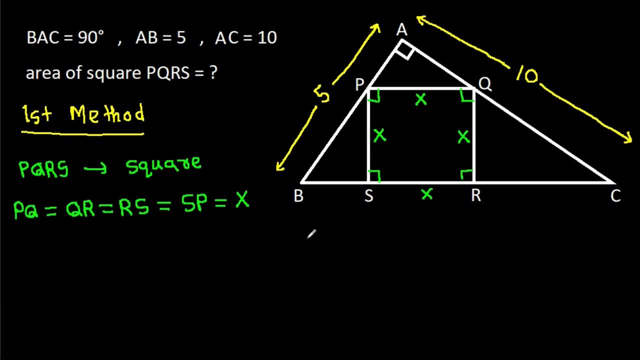 And now interangle ABC. this angle is 90 degree And suppose this angle is ANPHA, then this angle it will be 90 degree, minus ANPHA. Suppose it is BETA. so if this angle is ANPHA, then this angle it will be BETA And this angle it is 90 degree. 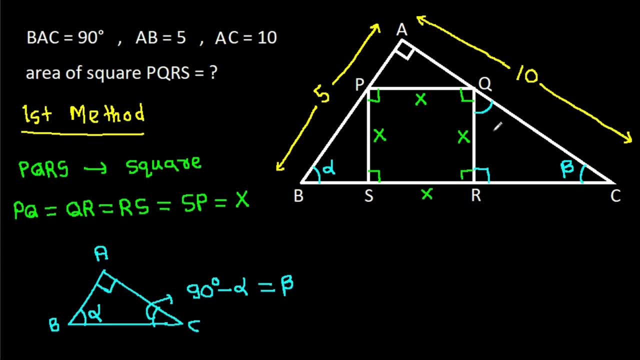 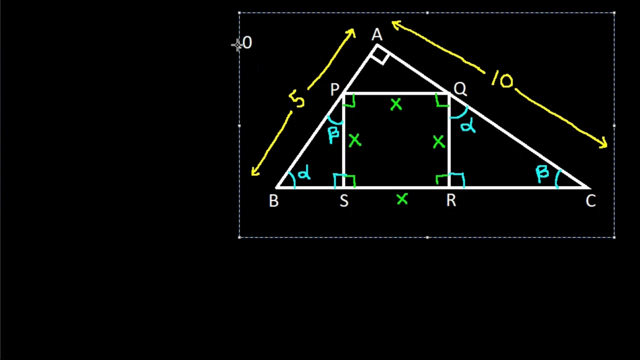 So this angle, it will be 90 degree minus BETA, that will be ANPHA. And this angle it is 90 degree. So this angle, it will be 90 degree minus alpha, that will be beta. and now in triangle ABC and triangle SBP and triangle RQC we have angle ABC is equal to angle SBP. 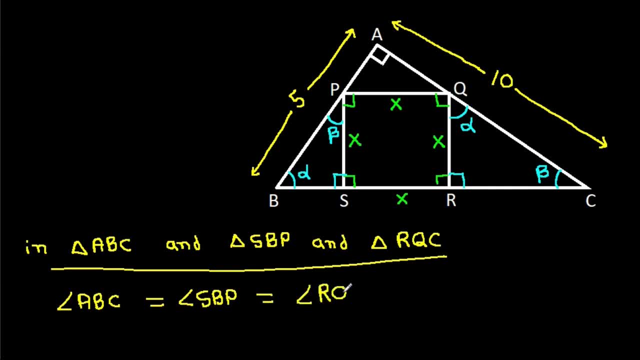 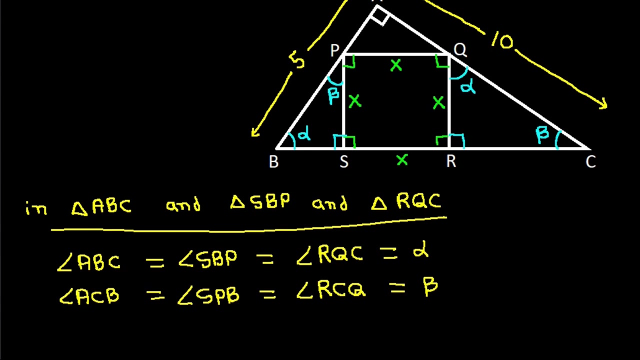 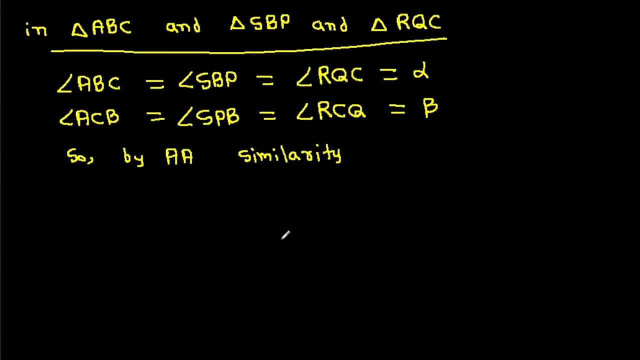 it is equal to angle RQC, that is alpha, and angle ACB it is equal to angle SPB it is equal to angle RCQ, that is beta. So, by angle angle similarity, triangle ABC: it will be similar to triangle SBP- it will be similar. 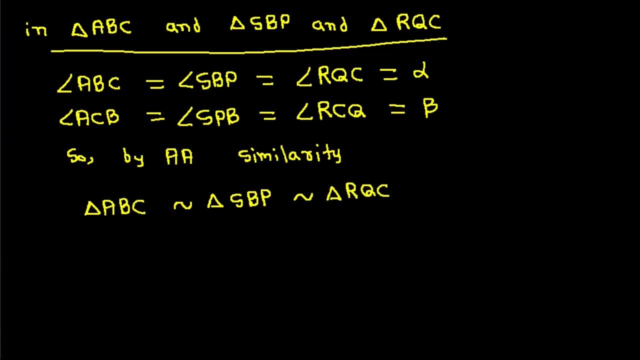 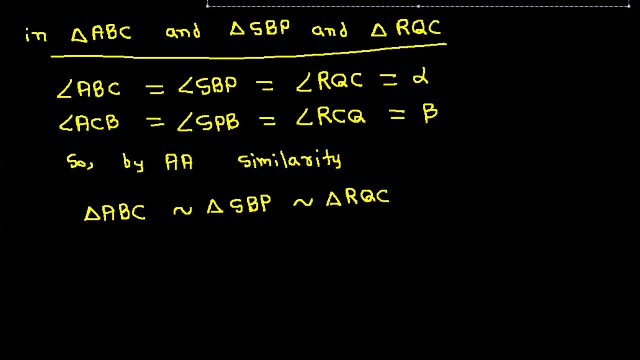 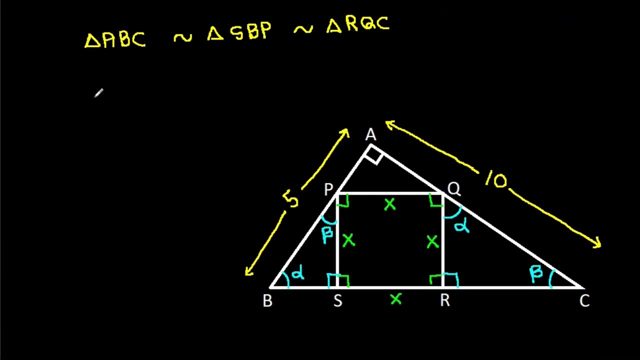 to triangle RQC. These triangles are similar, hence AB over AC. it will be equal to SB over SP it will. It will be equal to RQ over RC, and AB is 5 over SC is 10.. It is equal to SB over SP is X. 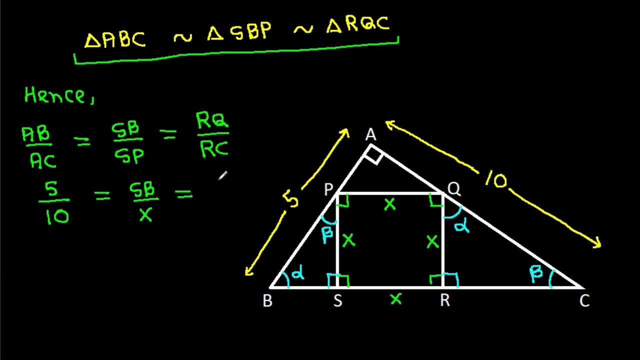 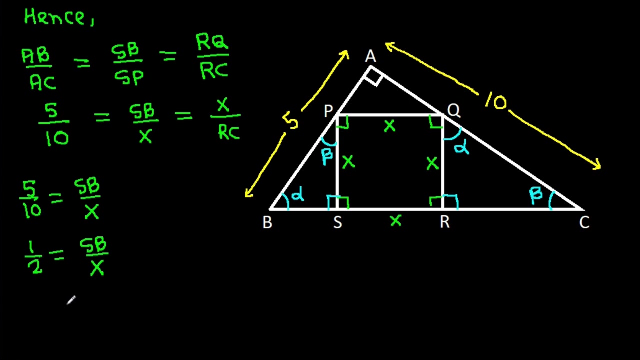 It is equal to RQ, is X over RC, So we get 5 over 10 is equal to SB over X and it is 1 over 2, is equal to SB over X, So SB it will be X over 2.. 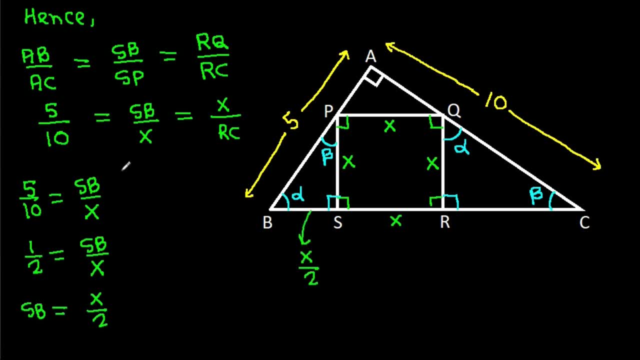 SB it is X over 2.. And also Now it is equal to SB over X, So SB it will be X over 2.. 5 over 10, it is x over rc, and 1 over 2, it is x over rc, So rc it will be 2x, rc it will be 2x. 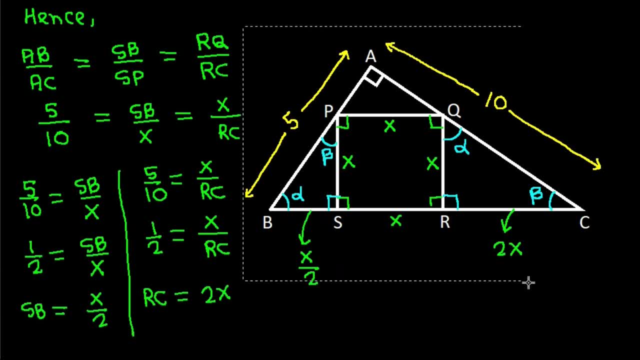 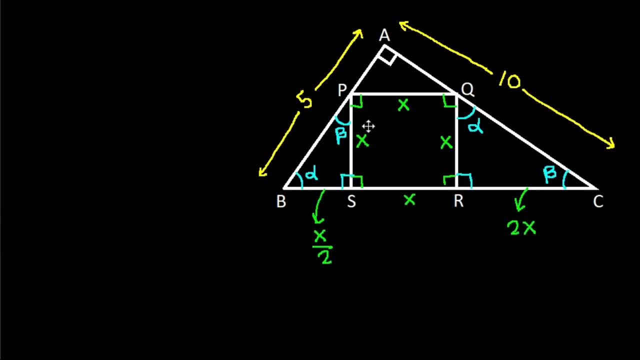 Now inter angle a- b is c, a- b is 5, a- c is 10 and this angle is 90 degree. So bc square it will be ab square plus ac square by Pythagoras theorem and bc square. 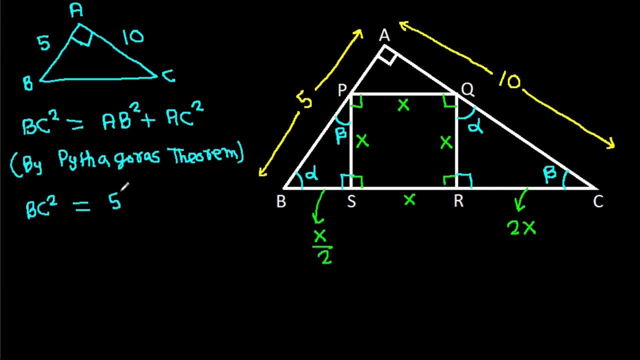 it is equal to: ab is 5 square plus ac is 10 square And bc square it is 25 plus 100, so bc square it is 125.. So bc it will be root 125, that will be 5 root 5.. 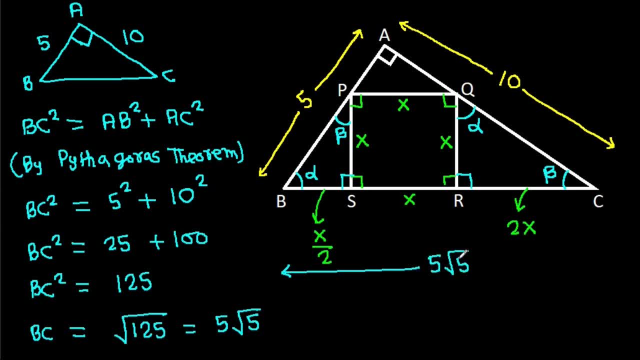 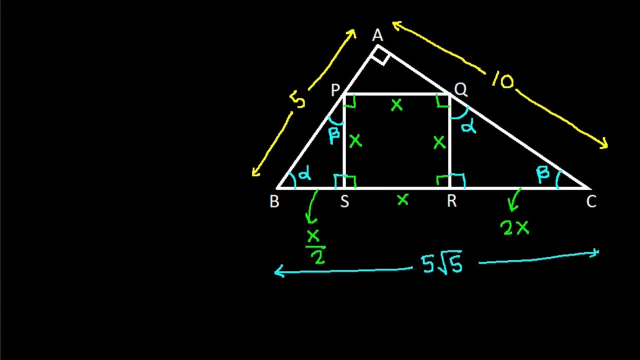 So bc, it is 5 root 5.. And now bc, it is bs plus sr plus rc and bc is 5 root 5, it is equal to bs is x over 2.. So bc, it is bs plus sr is x plus rc is 2x and 5 root 5, it is x plus 2x plus 4x over. 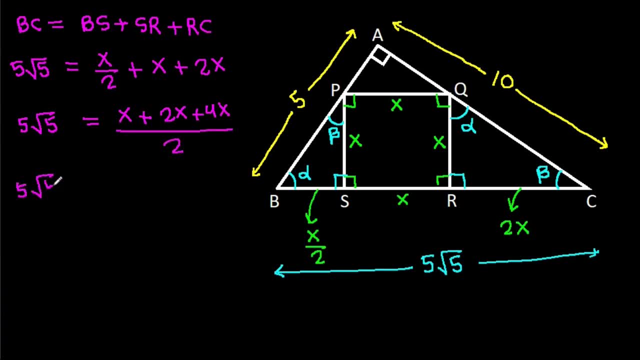 2 and 5 root 5, it is 7x over 2.. So x it will be 2 over 7 times 5 root 5.. So x it will be 2 over 7 times 5 root 5.. 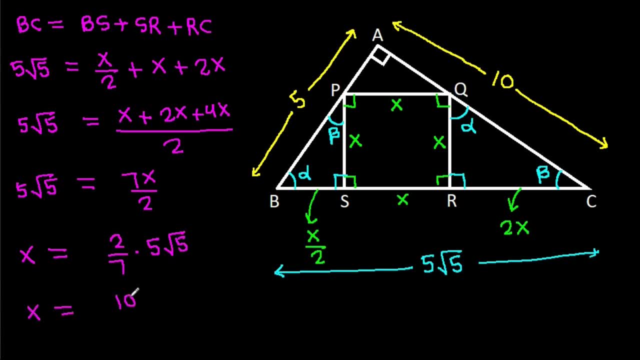 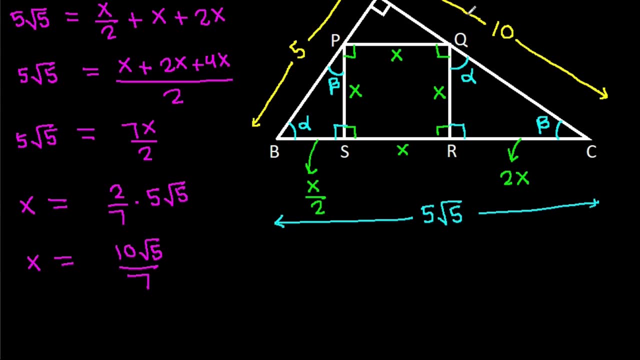 So x, it will be 2 over 7 times 5 root 5.. So x, it is 10 root 5 over 7.. And now area of the square pqrs. it will be side square and side is x square. 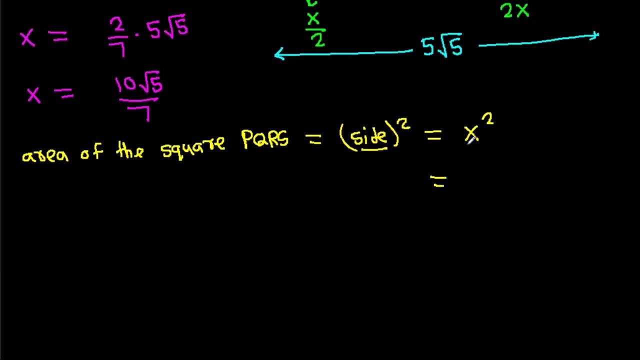 So x. it is 10 root 5 over 7. and now area of the square pqrs. it will be side square and side of the square and x is 10 root 5 over 7 square. So x is 10 root 5 over 7 square and it is 100 times 5 over 49.. 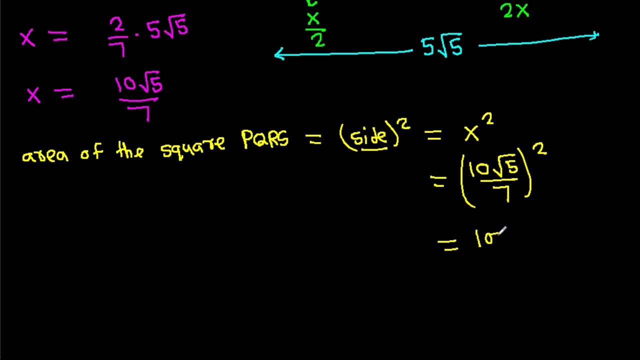 so x is 10 root 5 over 7 and it is 100 times 5 over 49.. That will be 500 over 49.. And this second method, Brach Viel, Warschild, mad션다, is two times 5 over 49.. 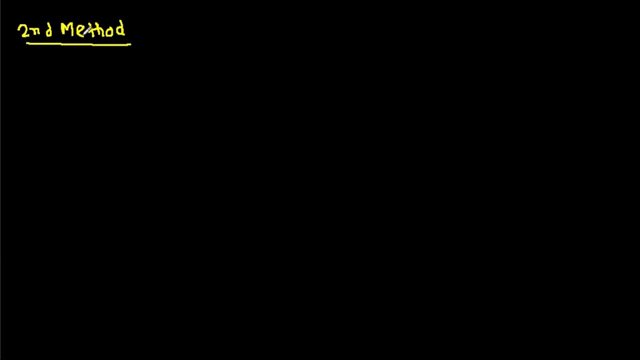 That will be 500 over 49. We have AB is 5 and AC is 10. and now from point A, if we make a perpendicular on PQ and BC, suppose this point is M and this point is N, then area of ABC, it will be equal to: 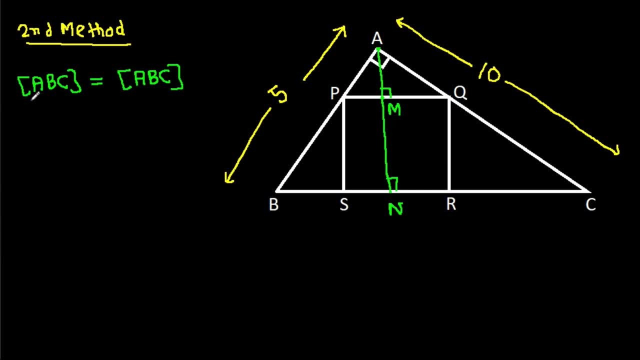 area of ABC. and area of ABC. it will be 1 over 2 times base is AB and height is AC. it is equal to. and area of ABC. it will be 1 over 2 times base is BC and height is AN. and 1 over 2 will get cancelled. and AB is 5 times AC is 10. it is. 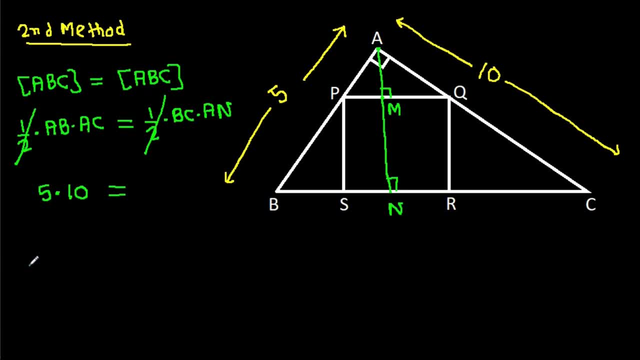 equal to And BC. it will be root under AB square plus AC square by Pythagoras theorem. so it will be root under 5 square plus 10 square and it is root under 125, that is, 5 root of AB square plus AC square by Pythagoras theorem. 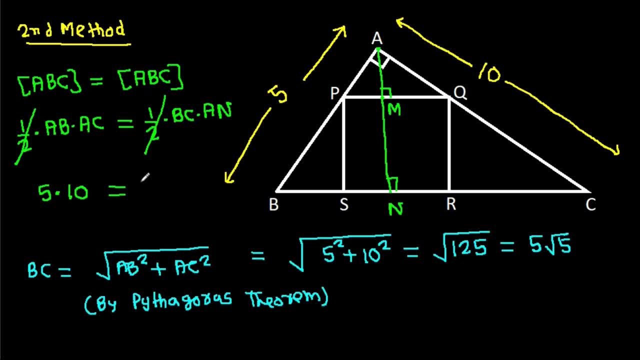 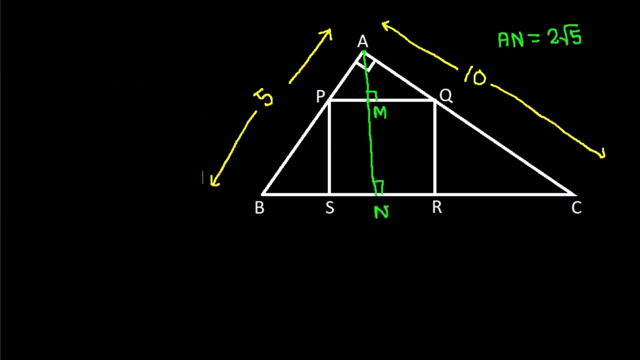 So BC it is 5 root 5 times AN and 5 will get cancelled. so AN it is 10 over root 5. that will be 2 root 5, we get AN is 2 root 5.. Now we know that PQ R S it is a square. so if PQ is X, then QR it will be X, SR it will. 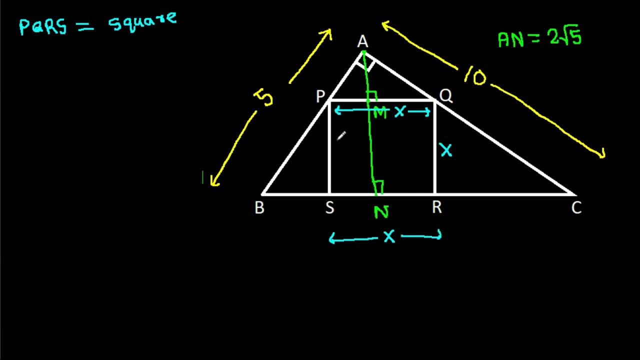 be X. So if PQ is X, then QR it will be X, SR it will be X, SR it will be X. So if PQ is X, then QR it will be X and PS it will be X and also SR it will be parallel. 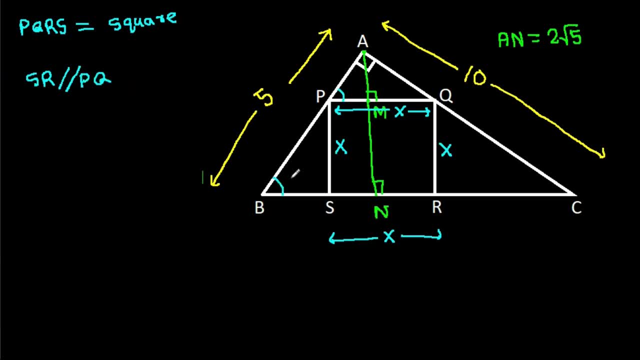 to PQ. that means these two angles, they will be equal. suppose AN, and these two angles, they will be equal. suppose BETA. So the angle of a形 is this: so AMB is same as 0 and 0 will be same as石RR is same as. 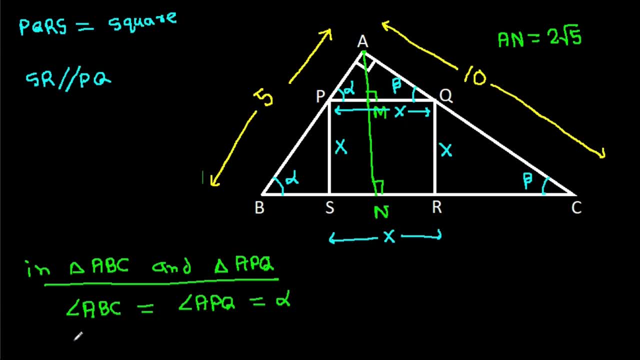 BC. that means both are equal. so becomes investigator twin element. So it will be VC, BC and RR To find it tilt, angle ABC and angle APQ. We have angle ABC is equal to angle APQ. that is alpha. it will be similar to triangle APQ. that means ratio of base BC over PQ. it will be equal. 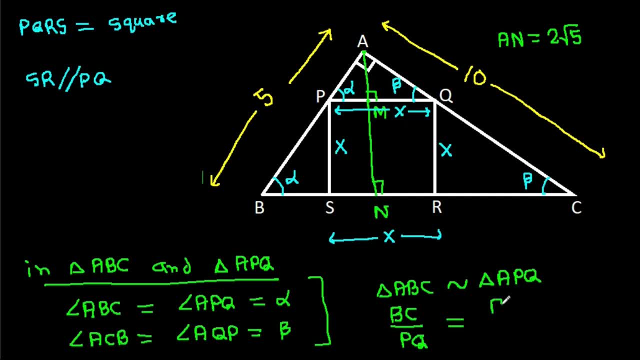 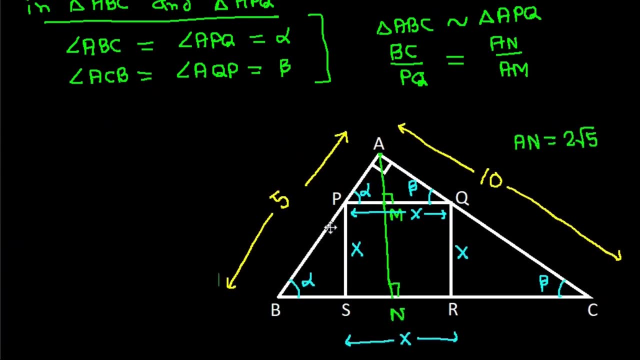 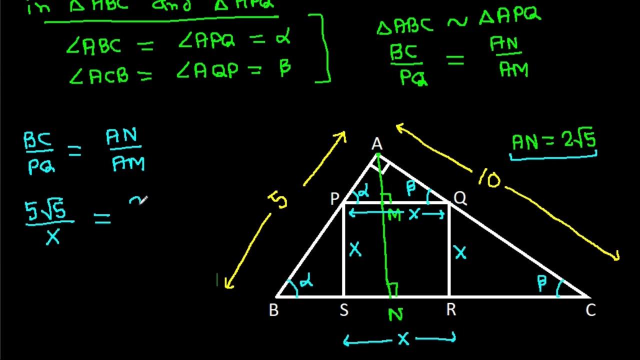 to ratio of height, AN over AM and we get BC over PQ is equal to AN over AM. Okay, And BC, it is 5 root 5 over PQ. it is X, it is equal to AN. it is 2 root 5 over AM. 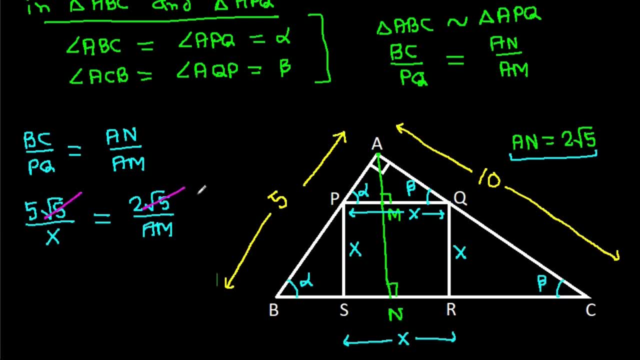 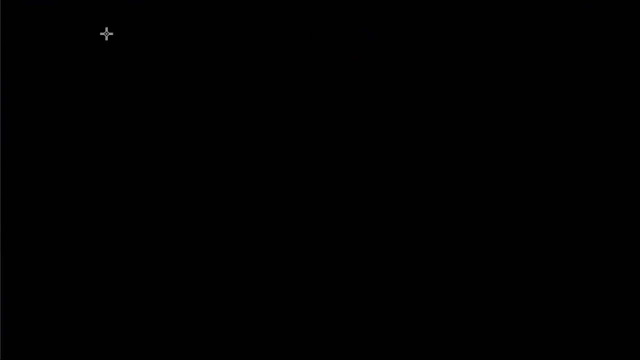 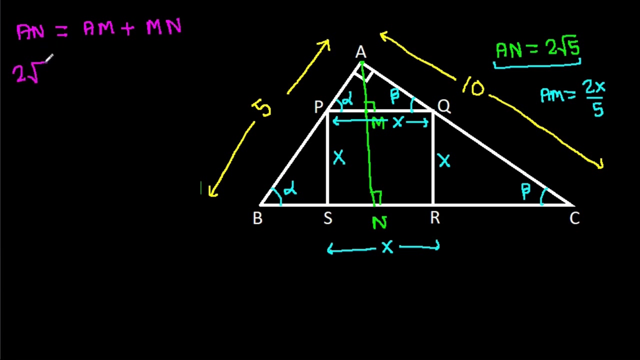 And root 5 will get cancelled, And so AM it will be 2X over 5, we get AM is 2X over 5.. And now AN, it is AM, AM plus MN and AN is 2 root 5, it is equal to AM is 2X over 5.. 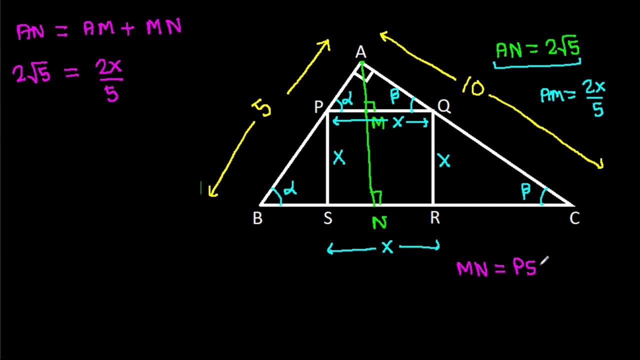 And MN, it will be equal to PS. that will be equal to QR, so it will be X. MN is X, So 2 root 5, it is equal to So 2X plus 5X over 5.. 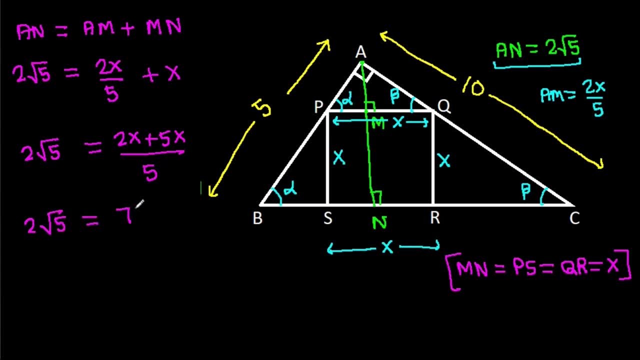 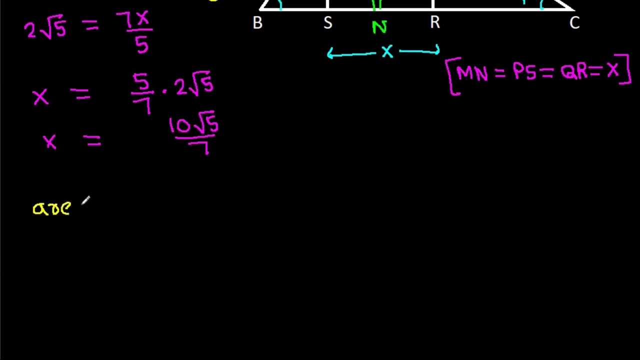 And 2 root 5, it is 7X over 5.. So X it will be 5 over 7 times 2 root 5.. So X it is 10 root 5 over 7.. And now area. 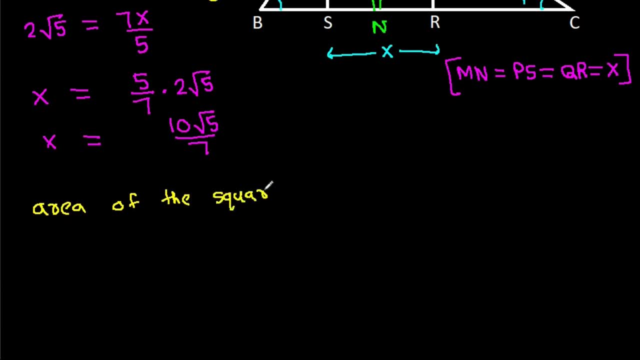 Area of D square PQRS. it will be X square, that will be 10 root 5 over 7 square and it will be 500 over 49..